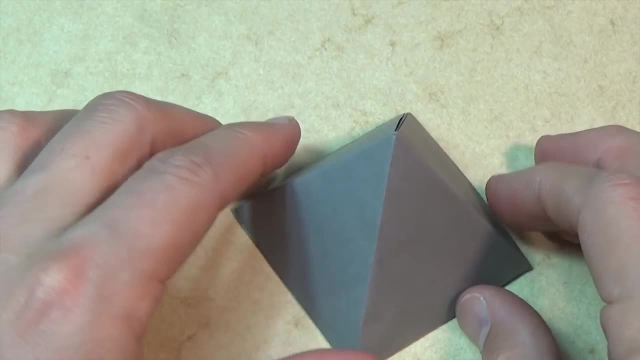 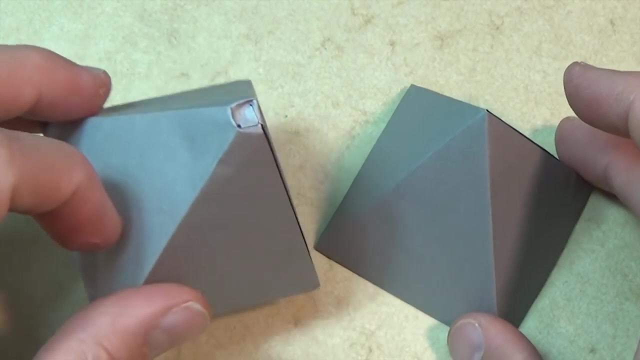 Hey guys, what's up? Jeremy Shaver here Today I'm going to show you how to fold this pretty easy, seamless pyramid. It's a new pyramid that I just designed, and I'm also going to show you how to make a dent in the top of the pyramid. Why would 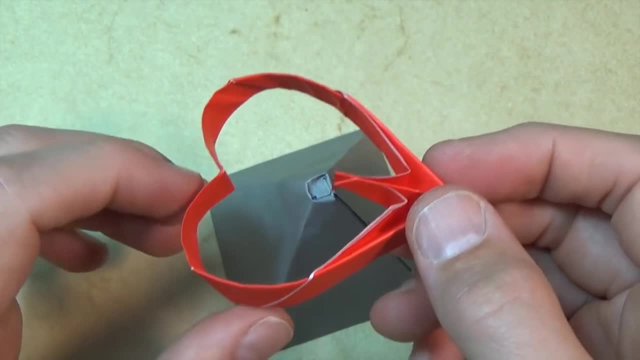 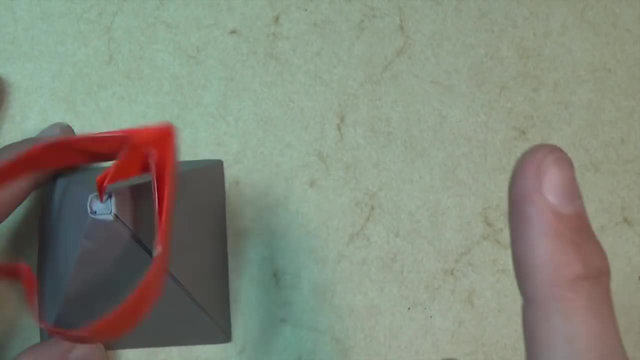 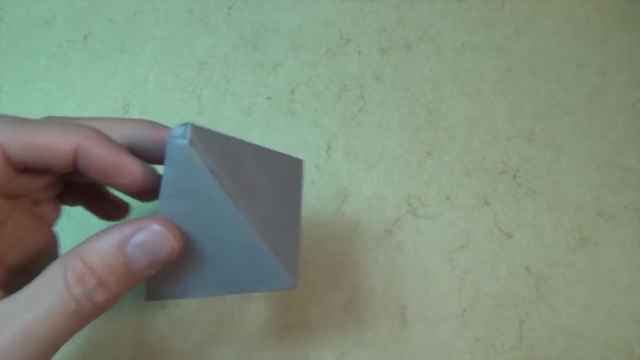 you want to make a dent So that you can balance this heart bird on it and spin it. For the heart bird, I made a separate tutorial here for the pyramid Ready set. here goes Alright. so to fold this model, I'm going to use a six inch square of. 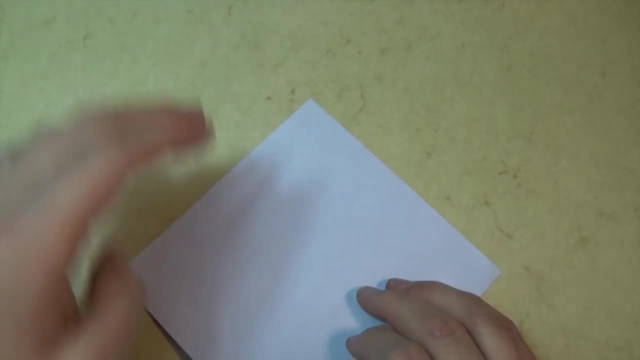 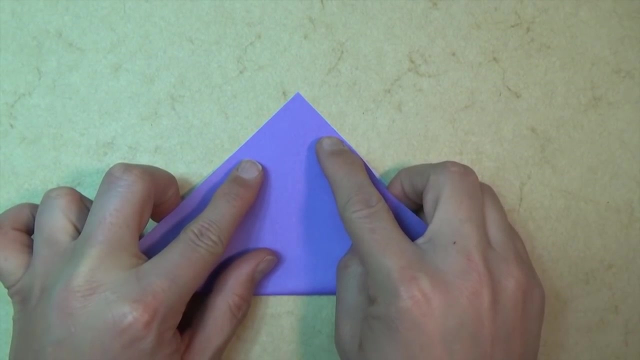 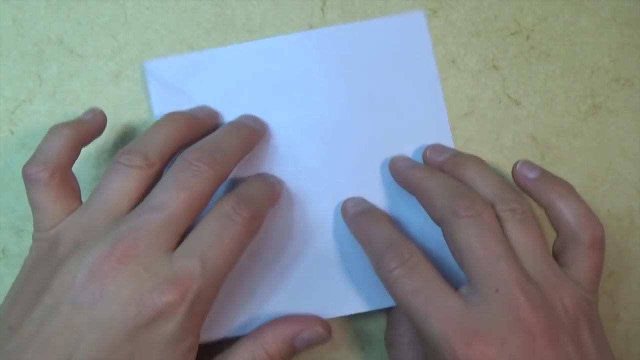 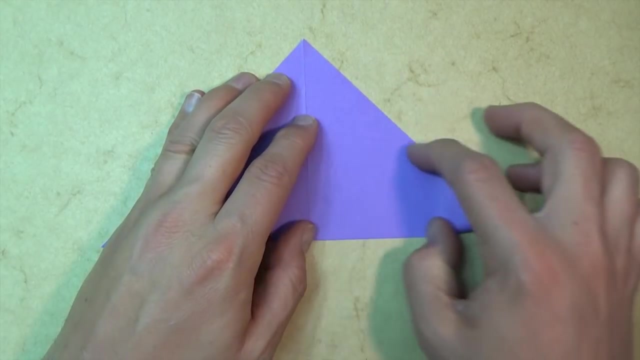 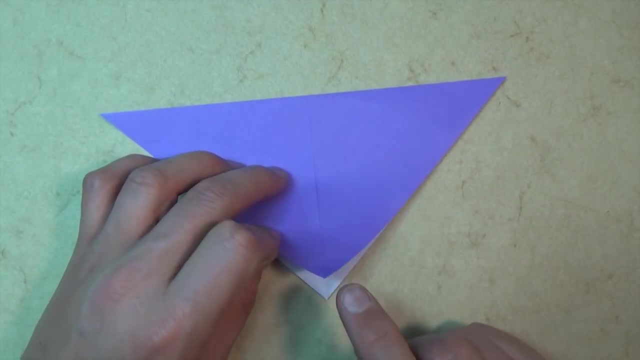 commie, and let's begin white side up and let's valley, fold diagonally in half. Try to make really precise folds and crease sharply. Now let's unfold and rotate, and let's fold in half in this direction. Okay, let's rotate again. And now let's fold just the top flap so that this corner 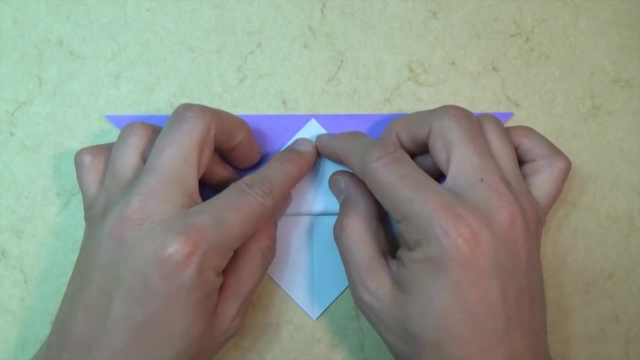 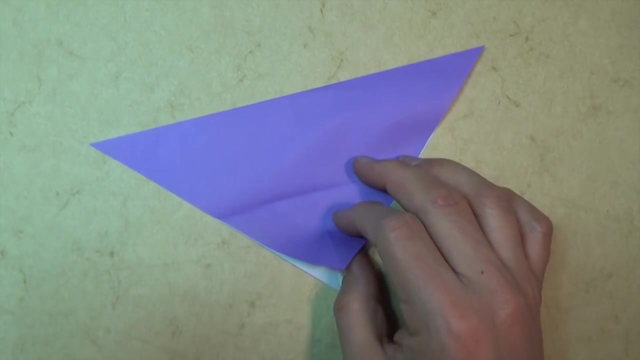 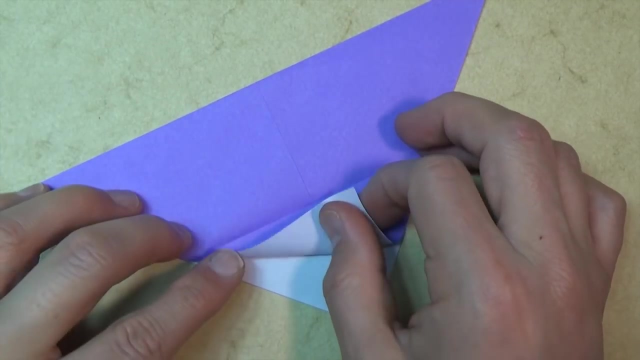 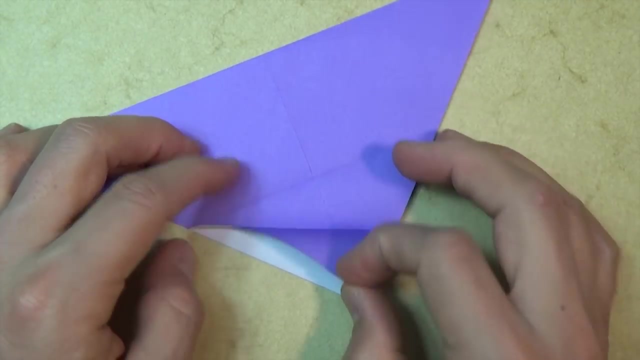 touches this point right where the crease hits the edge, Like that, And let's unfold. And now let's fold the flap so that this edge aligns with the crease, And unfold, And let's do the same thing on the right. So let's fold it so that this: 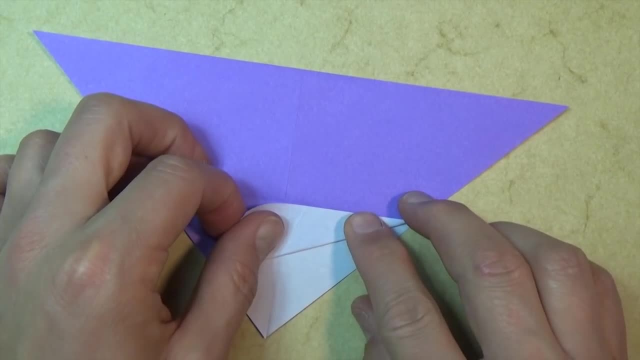 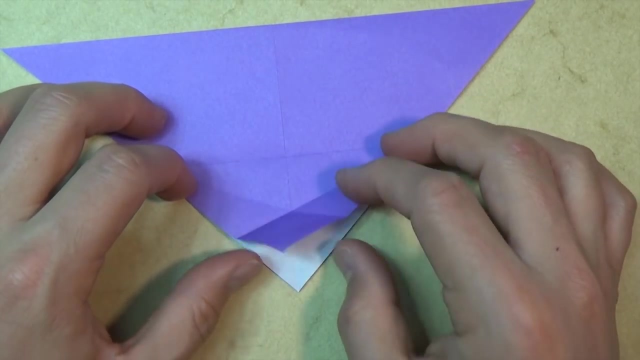 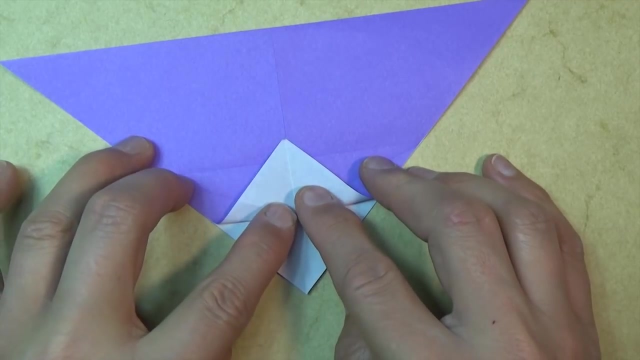 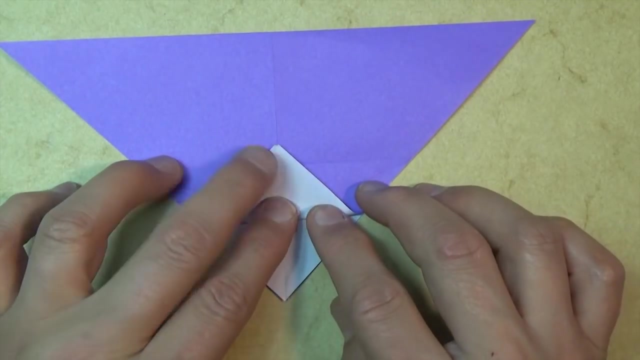 edge aligns with the crease And unfold. And now let's fold the flap up right on this point And when you fold it up, you want this crease to align with this crease And this crease to align with this crease. 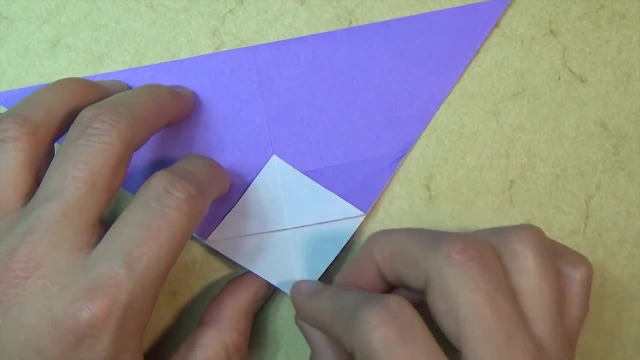 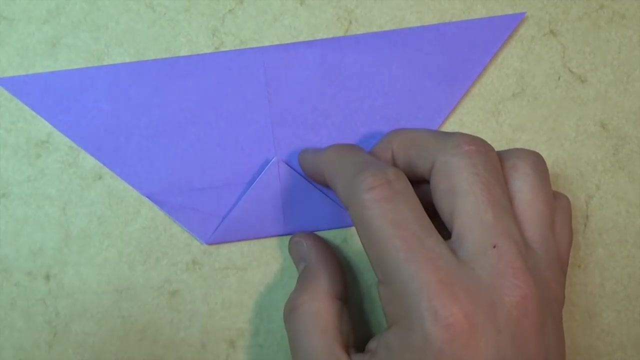 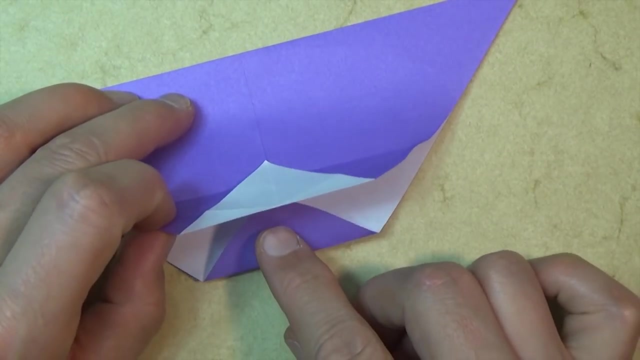 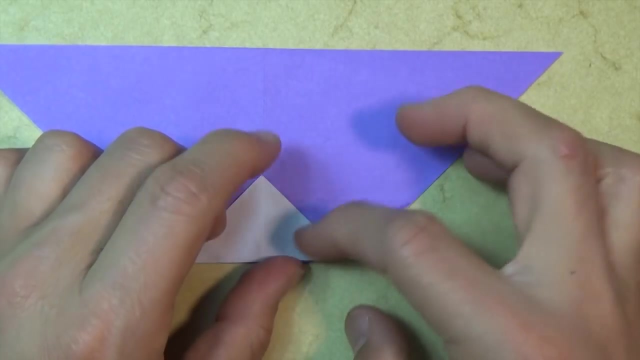 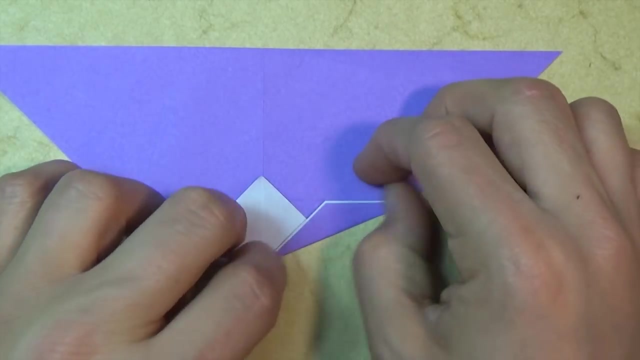 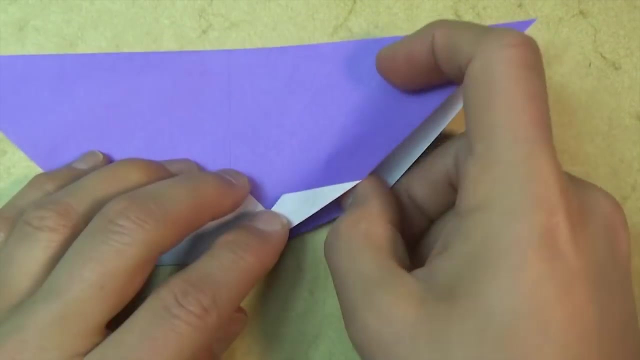 Okay, And now let's fold this flap up right on this edge And unfold the top flap And refold it, sticking it underneath, Like that. Okay, Now let's fold right on this crease, Fold on all layers, Like that, And let's unfold the top flap and stick it underneath And let's do. 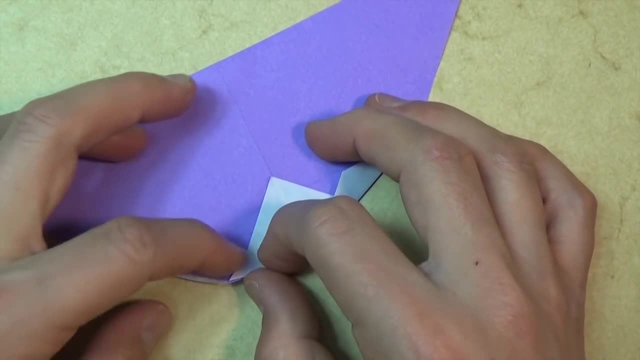 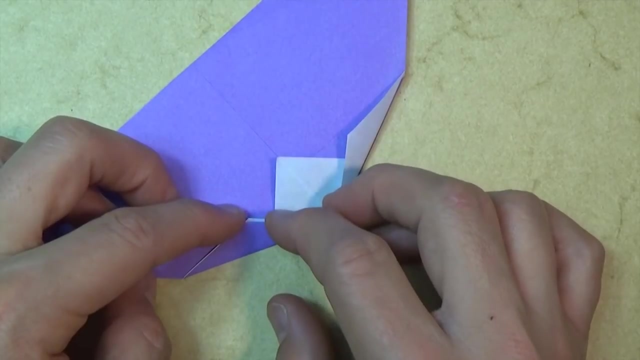 the same thing over here. So let's fold on all layers on this crease And unfold it, And then like that, And unfold, And like that And unfold. We don't have to stop for. unfold the top flap and refold it, sticking it underneath. 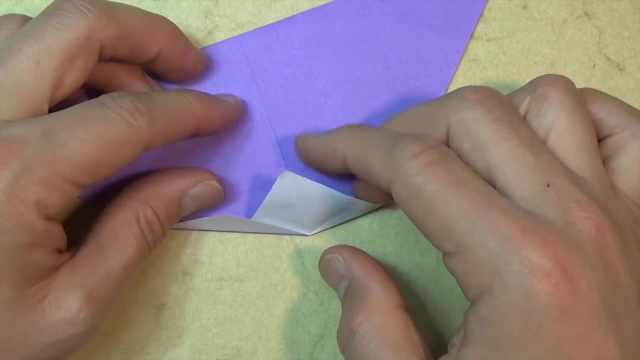 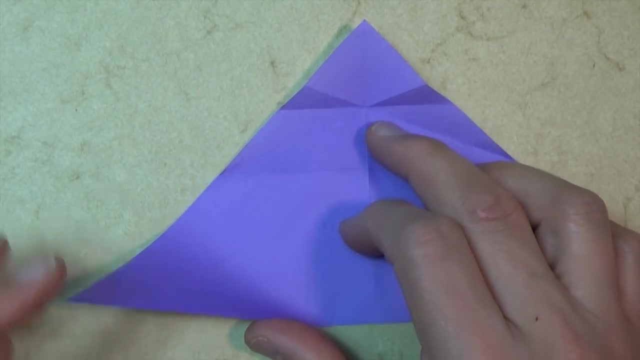 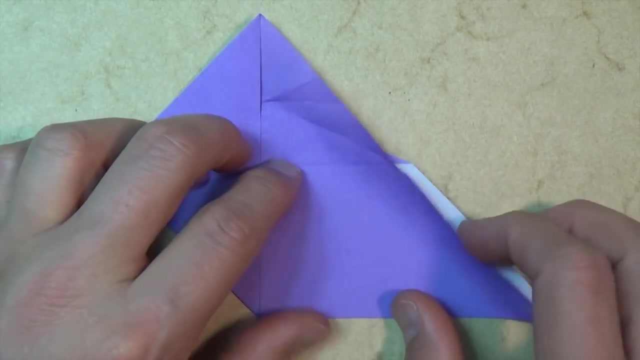 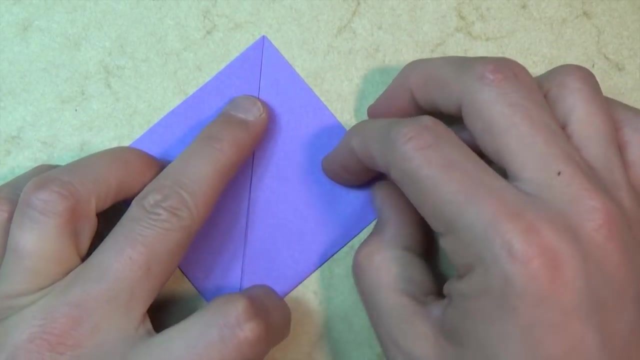 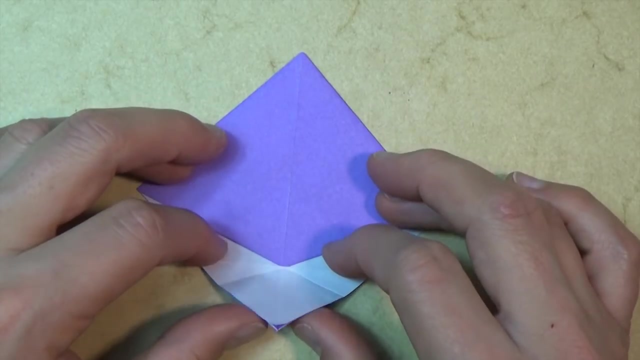 Okay, now let's unfold this flap and rotate and let's fold this corner to this point And let's do the same thing here. Let's fold this corner to here And let's turn over top to bottom And let's fold right on this horizontal crease. 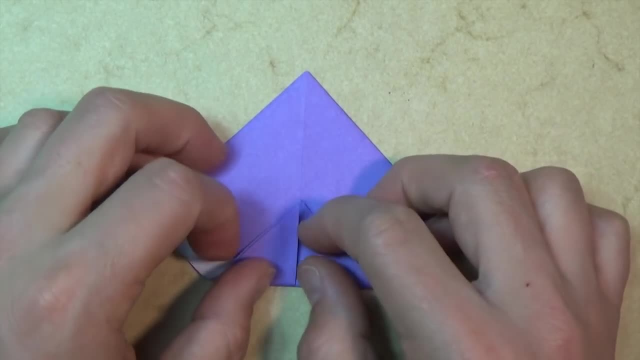 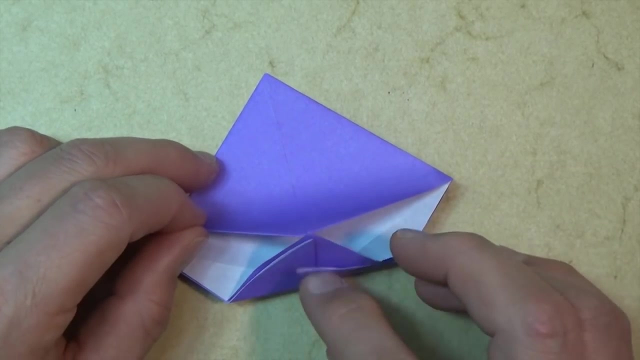 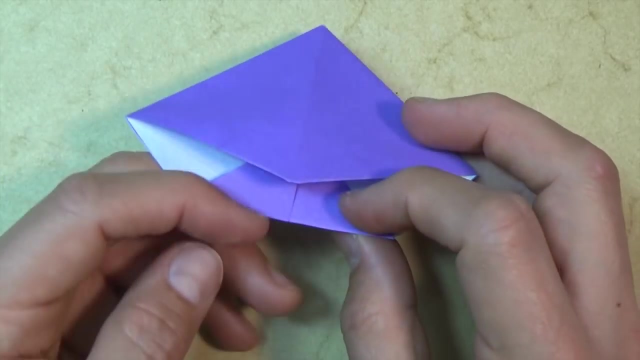 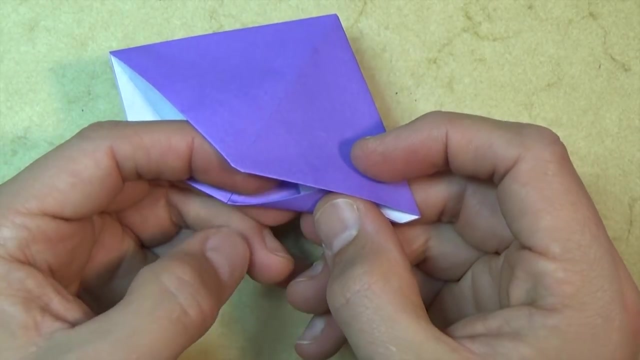 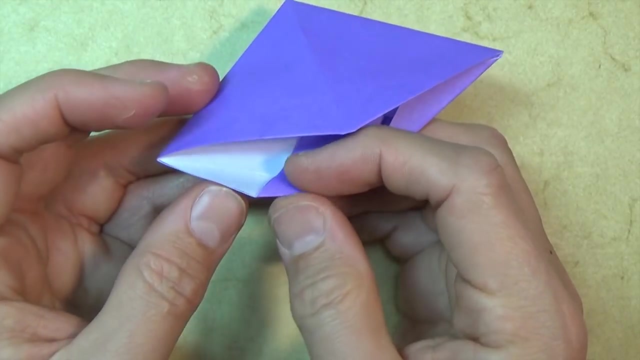 So we're just folding all layers just up like that And let's unfold them and refold them, sticking them underneath. And now let's fold this flap in right on this existing crease And same thing on the left side. Fold this flap up on this crease. 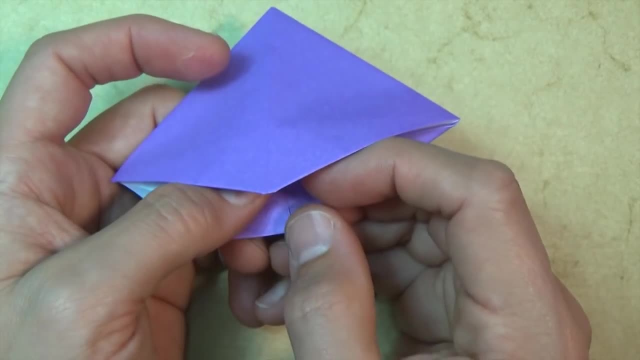 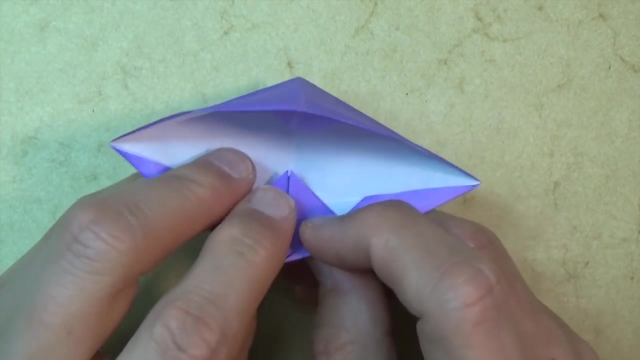 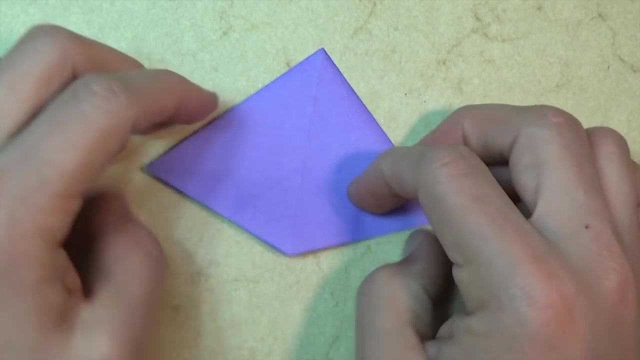 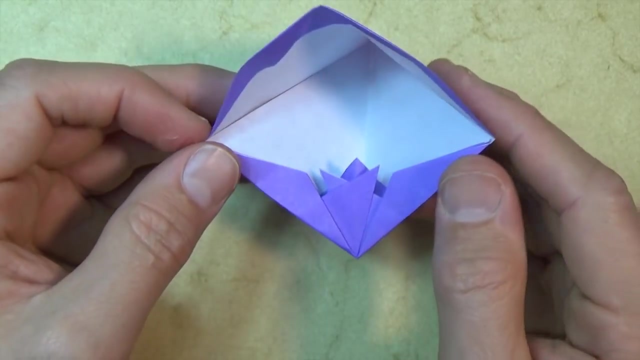 And fold it to the pocket. Try to make it so that these flaps stay together when you make that fold. So it's like that And flatten. Okay. so here we have the pyramid to be. Let's open this flap and just 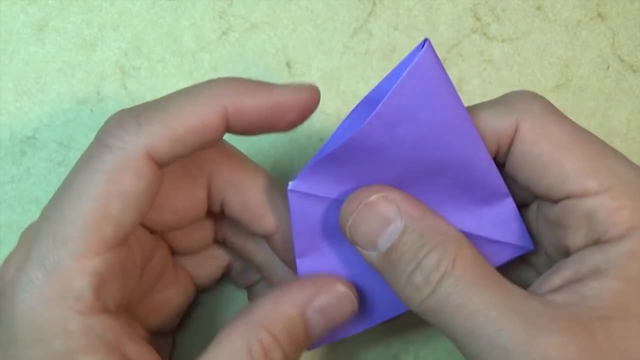 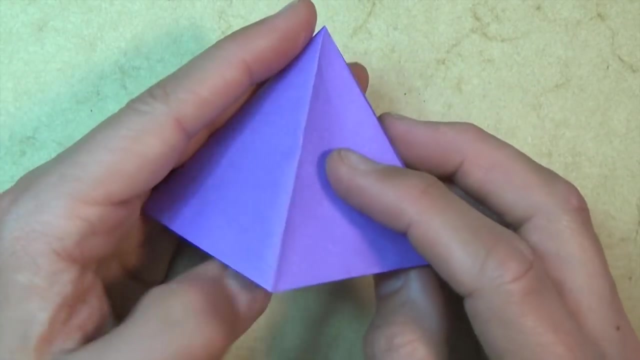 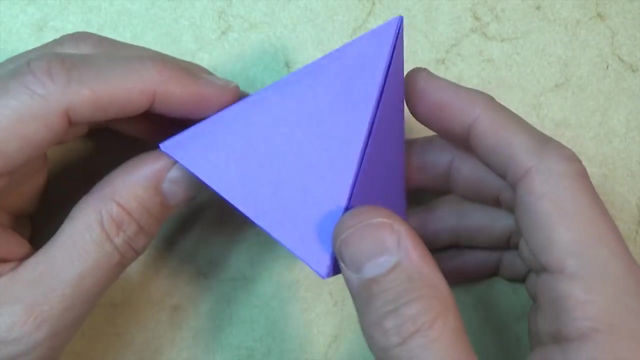 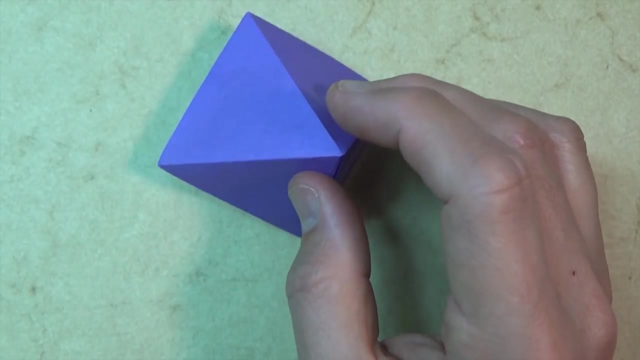 bring these two corners together, kind of like a cootie catcher, And go back like this and do that a couple times And here we have the pyramid. Okay. so if you like it like that, then you're all done. But if you want to make the dent in the point so that you can balance a bird on it, 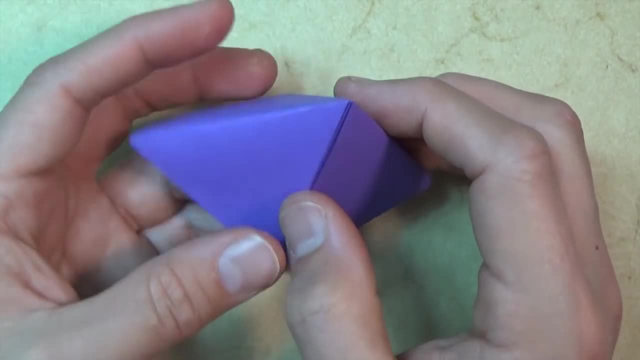 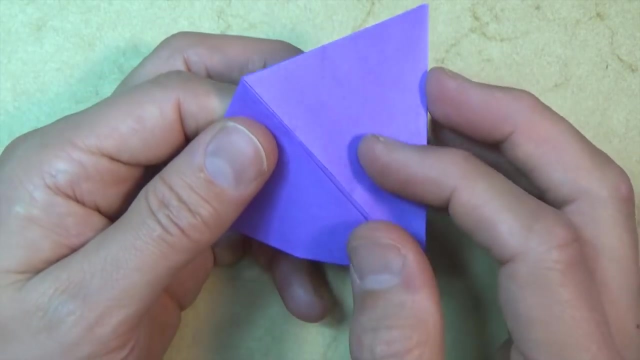 well, it's hard to balance it like that, so you really need to make the dent. So here it goes. Let's rotate and flatten it so that you have these edges right here. These edges are on the front. And now let's take this. 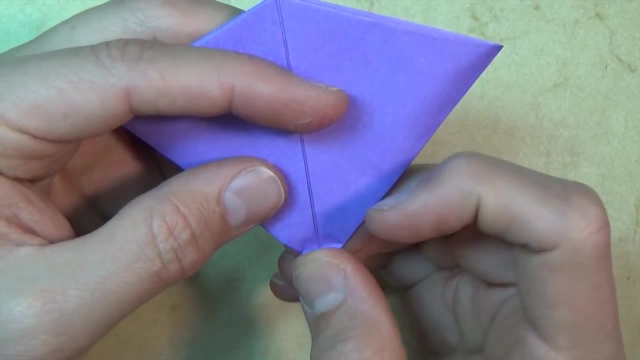 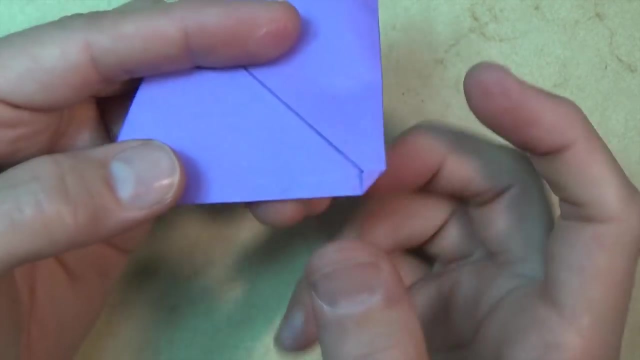 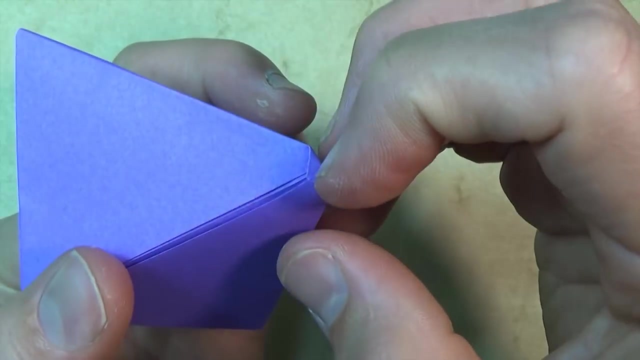 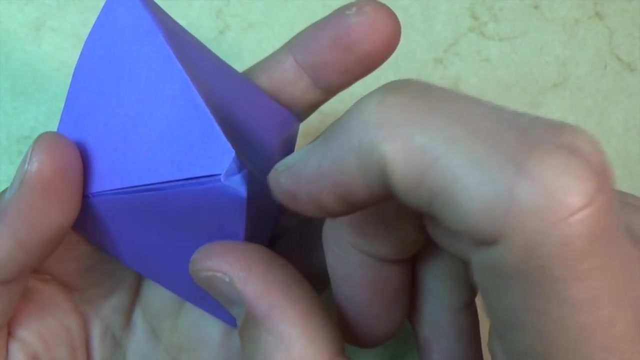 this point and just fold it up just a tiny bit. so it's like that. okay, and now stick your finger into the pocket and you want to put your fingernail right on the existing crease and just push it down like that your other finger should. 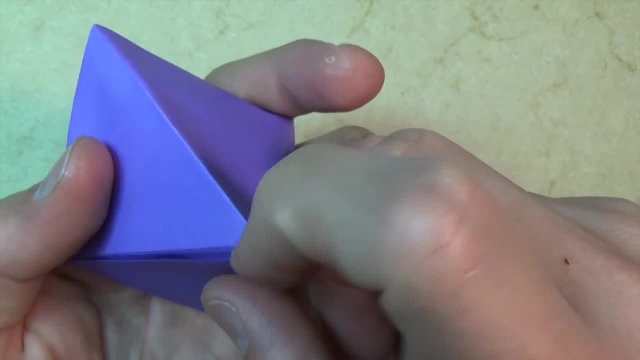 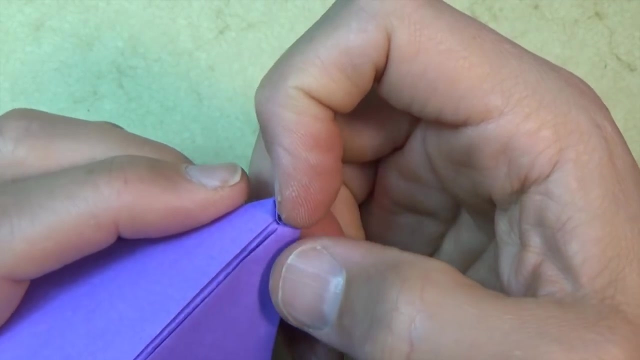 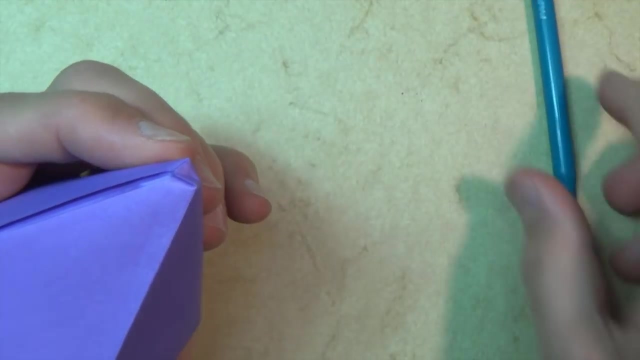 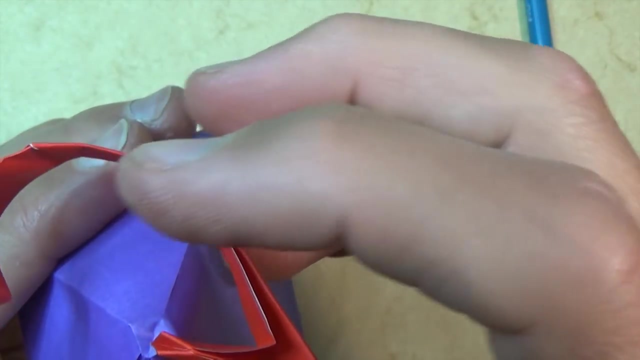 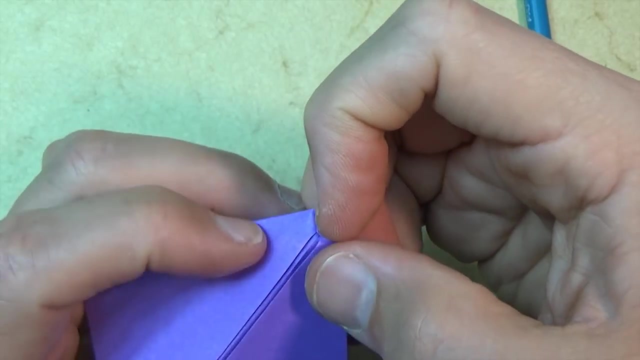 be all the way inside and just press it down. you want to press it so that you end up with two, two peaks, one and two, and even right here the bird could balance. but we're gonna do something to make it even better. it's better. so here we have the two peaks. what you want to do is take a. 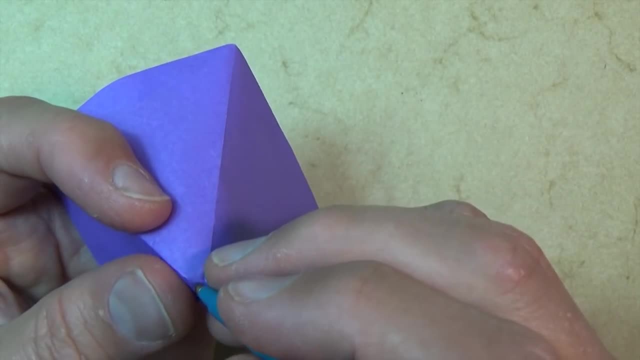 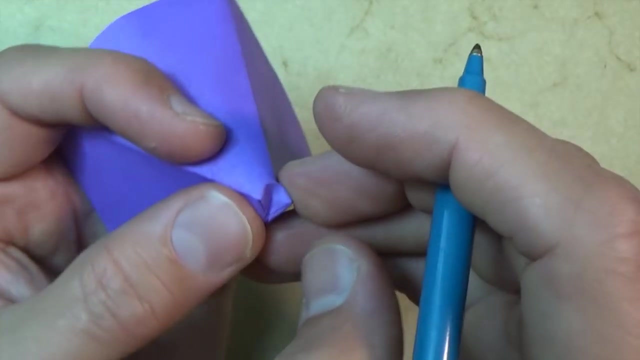 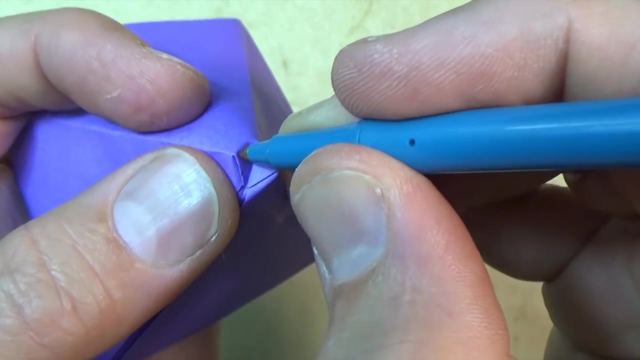 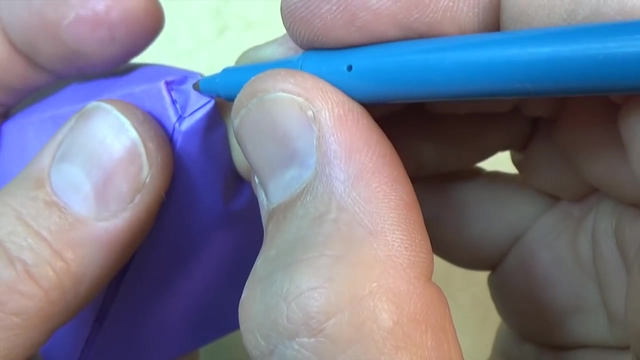 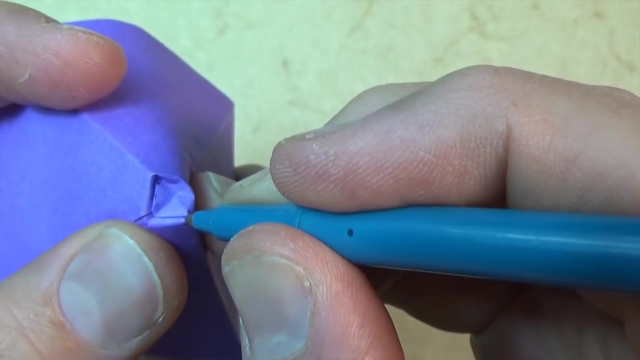 ballpoint pen or some other sharp object and you want to press, you want to press right on the peaks, right on the corner. so just press right here and just push that point down down like that, and do the same thing with this peak, just get it so with. it is right, kind of on the inside of the peak, right there, and 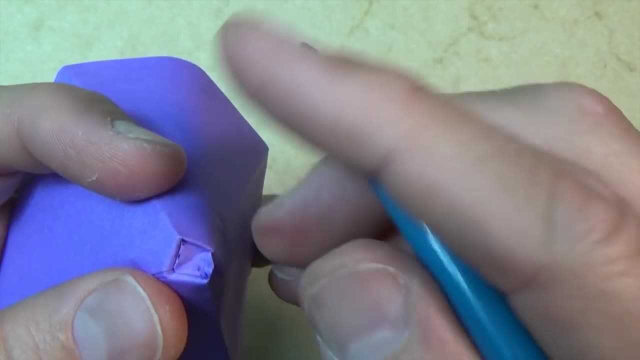 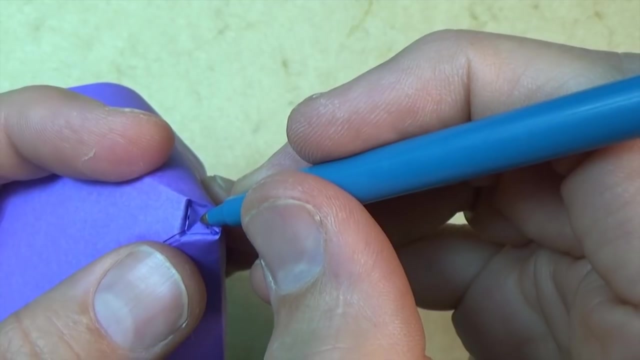 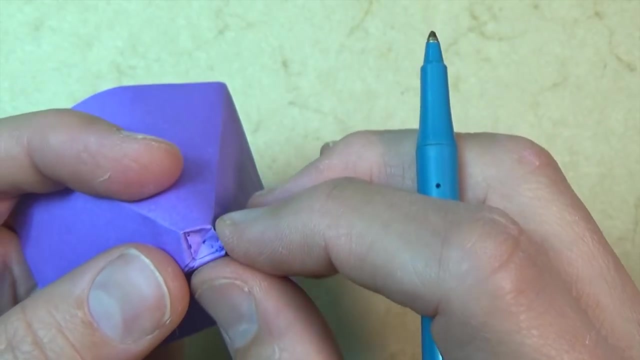 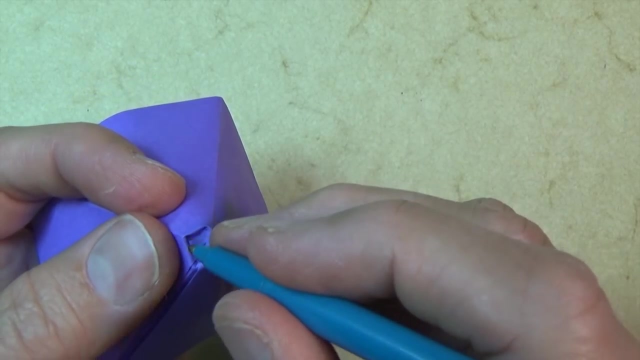 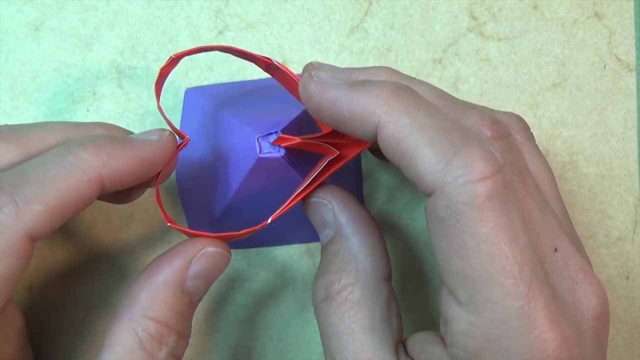 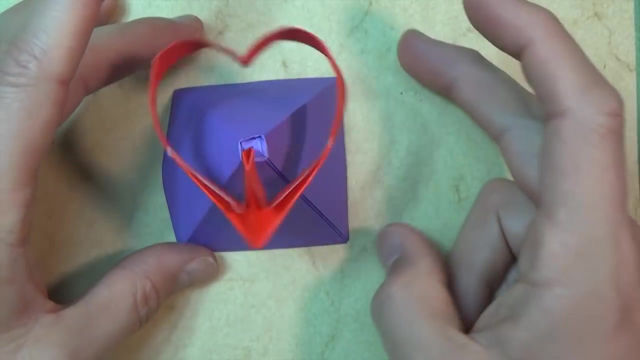 just press it down like that, and that way you end up with a little indentation right here. this should you go down so that that's where the bird will balance, And ideally this right here should be square, so it's like that. And now the bird balances right on the middle and it spins.